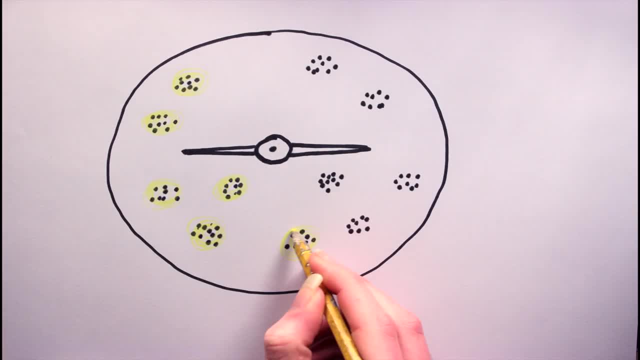 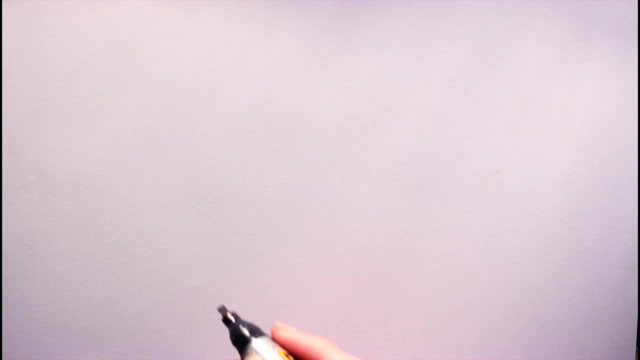 Spiral galaxies form in this disk and objects resembling spherical collections of stars live in this halo. These collections are known as globular clusters, and they tend to orbit around the galactic core. Encasing the halo of stars is yet another halo that extends huge distances into the cosmos. 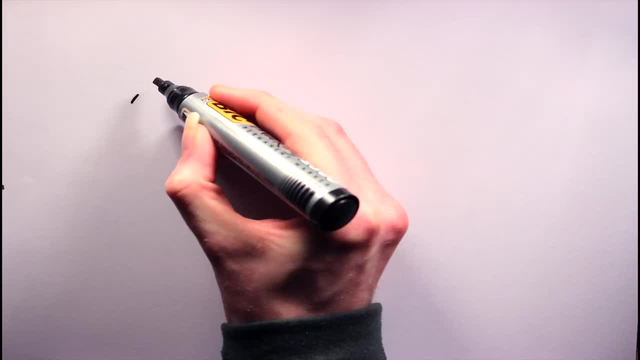 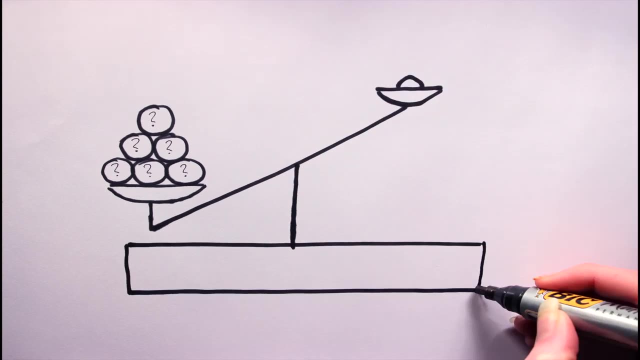 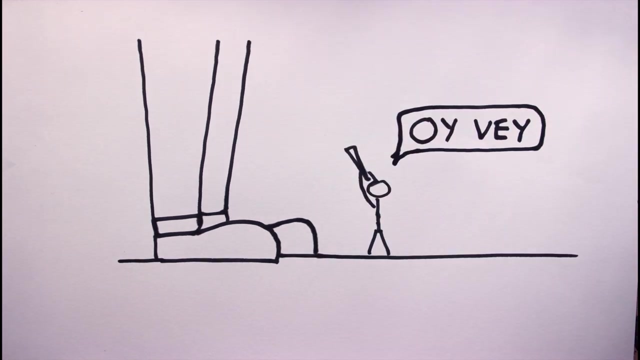 This halo is comprised solely of dark matter. It is estimated that 95% of the mass of a galaxy is made up of dark matter. Or put another way, when we look at a galaxy, we are only seeing 5% of its structure. Galaxies are much bigger than is immediately apparent. The distinctive spiral. 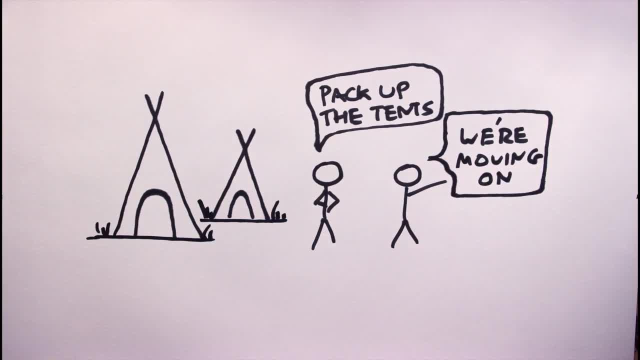 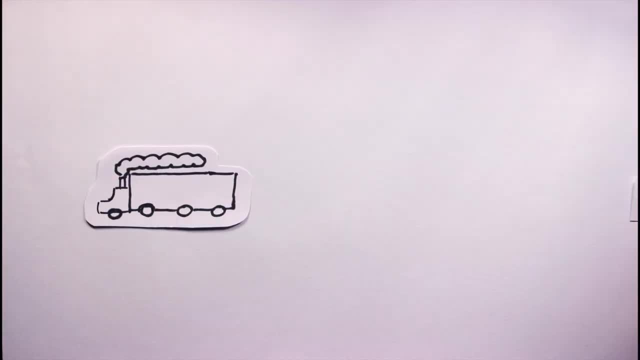 arms that extend out from the central region of the galaxy are not permanent structures. The pattern we see is, in fact, a density wave. Think of a density wave as a cosmic traffic jam. Free moving cars- or matter in this case- will bunch up at the scene of the jam but slowly return to 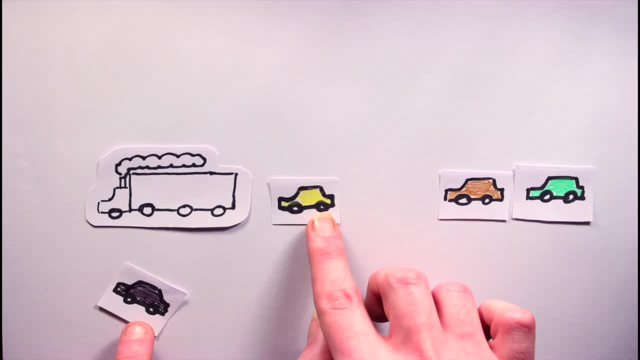 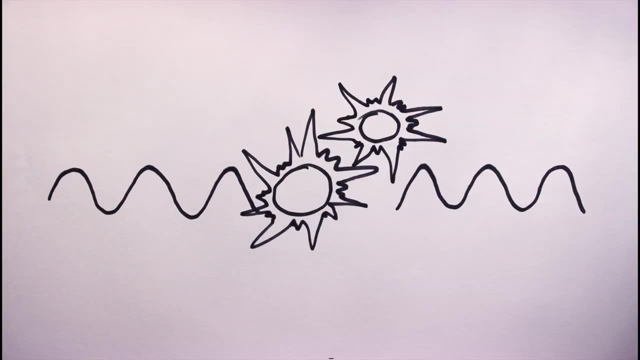 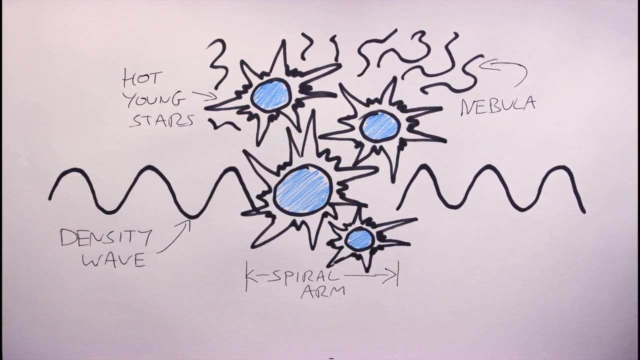 normal speed as they pass the obstruction. The result is a moving traffic jam which stays constant but never involves the same cars. Galactic bars rotate around the galaxy, interact with the interstellar medium and trigger star formation, resulting in the creation of nebulae and hot young OB stars. It is these OB stars. 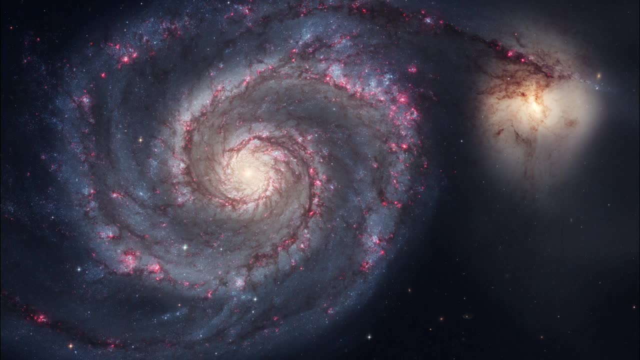 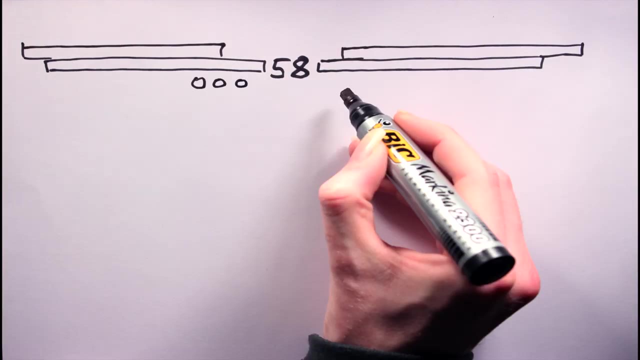 that give the spiral arms their bluish colour. The nebulae that dot the arms tend to glow red, and any dark streaks and patches are lanes of gas and dust. Galactic bars are thought to be relatively short-lived and may form as a result of instabilities in the galactic disk or when two 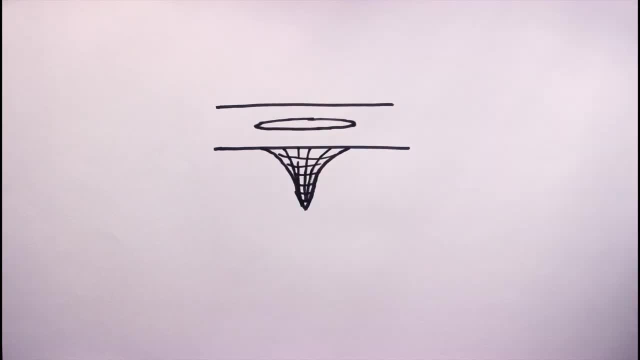 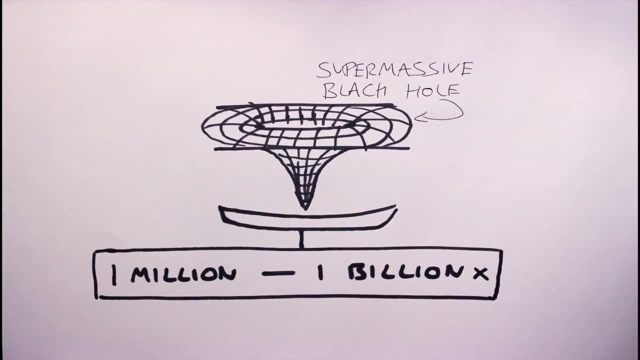 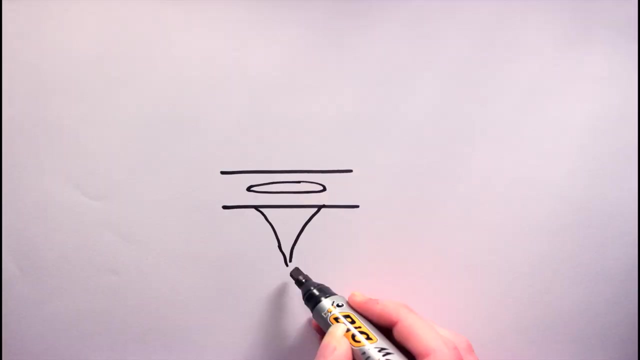 galaxies collide. Therefore, the central region, or bulge, hosts the supermassive black hole. A galactic supermassive black hole can have a mass of anywhere between a million and several billion solar masses. A galaxy can either be said to be dormant or active. In an active galaxy, the supermassive 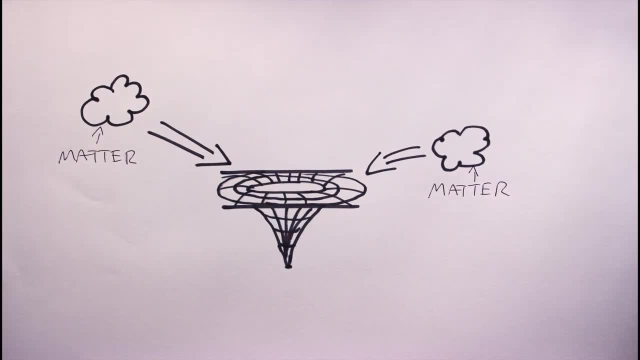 black hole at the centre regularly gobbles up material and, as a result, ejects high energy particles into intergalactic space. Depending on the type of emission, these galaxies can be referred to as starburst, quasar and starburst. 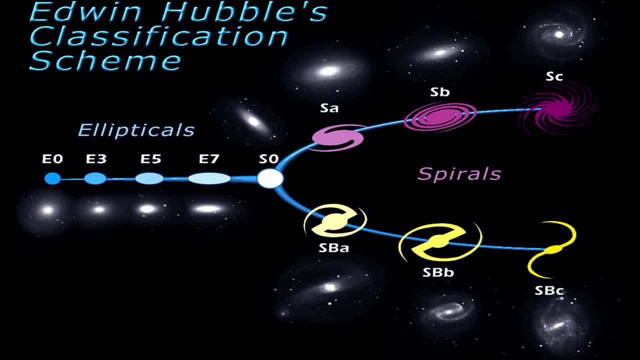 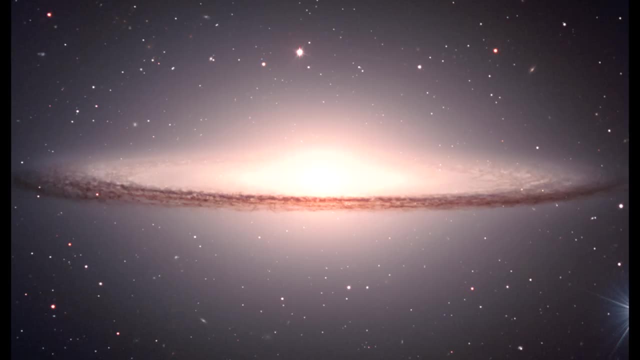 Let's look at the Hubble tuning fork diagram. Here we see that spiral and barred spiral galaxies come in a variety of different shapes. They are defined based on how loosely the arms are packed and how big the central region is. Finally, I'm going to leave you with some examples of spiral galaxies.